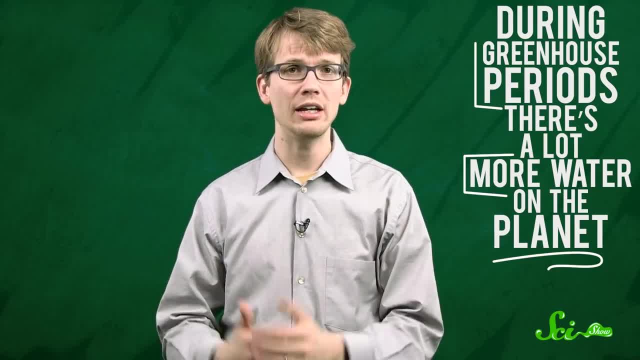 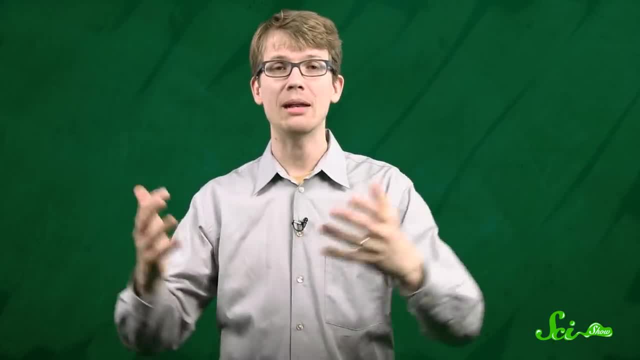 During greenhouse periods, there's a lot more liquid water on the planet and very little, if any, ice at the poles. During icehouse conditions, the global climate is cold enough to support large sheets of ice at both the poles. The most recent transition between these two is the global climate. 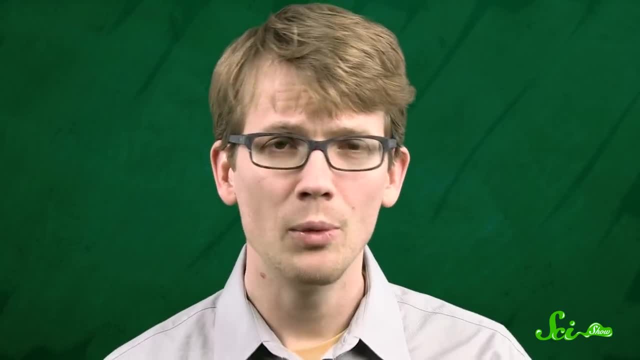 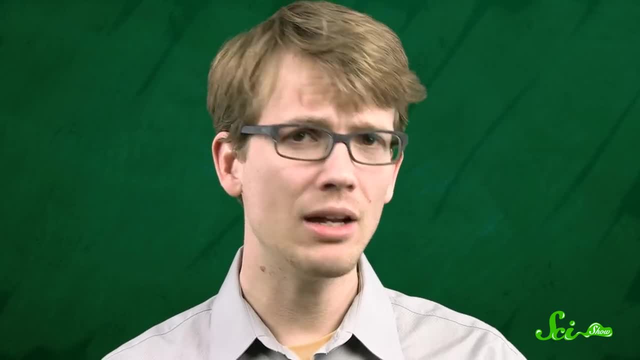 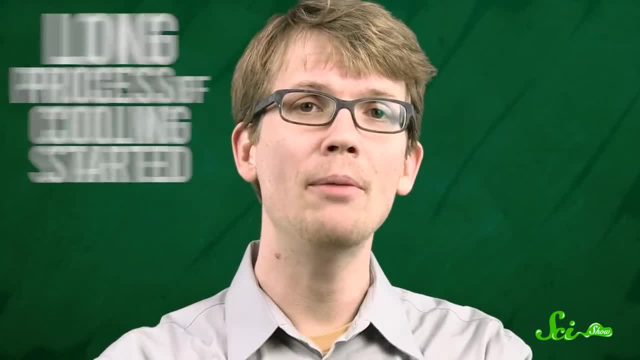 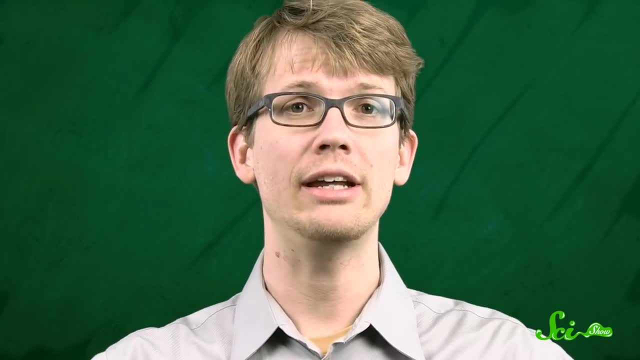 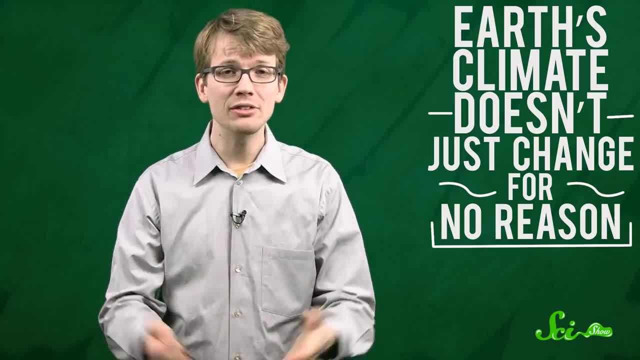 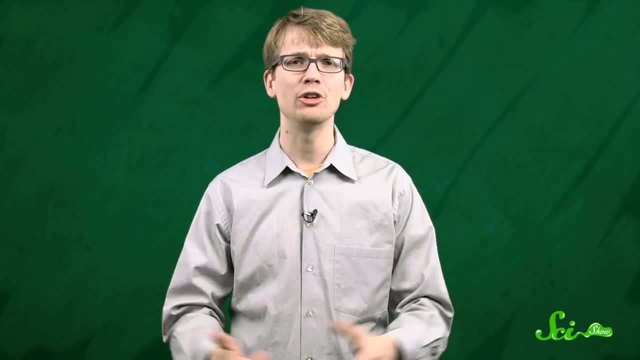 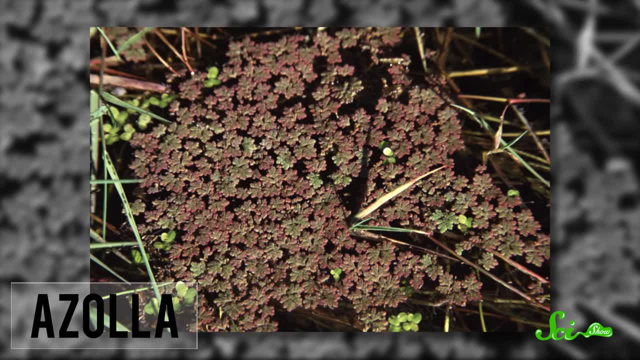 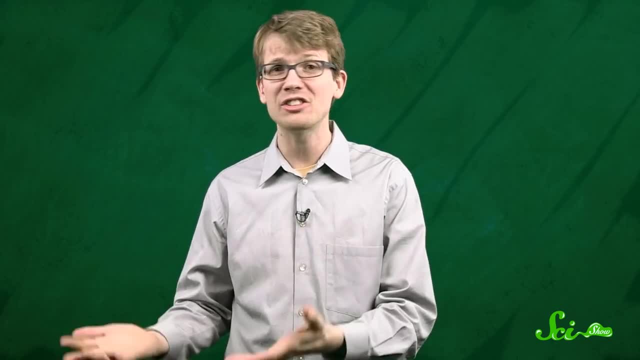 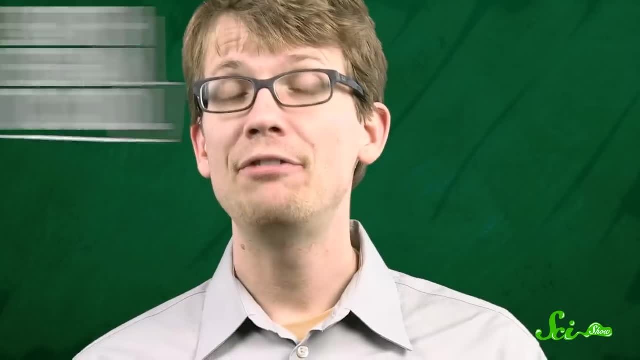 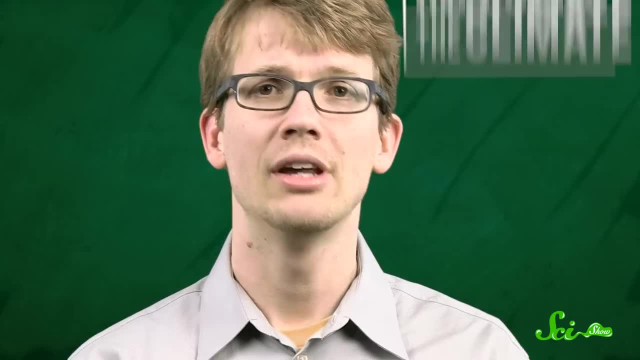 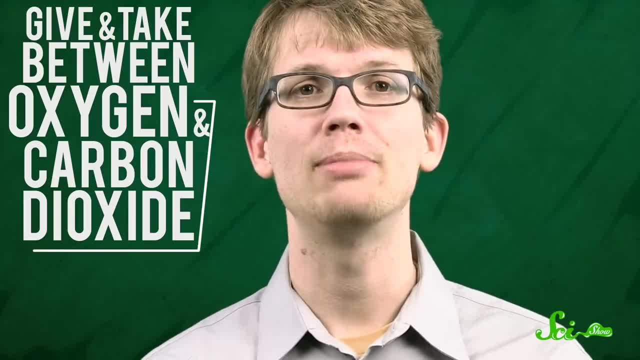 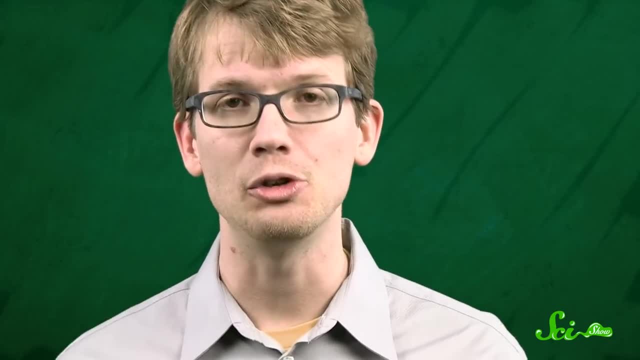 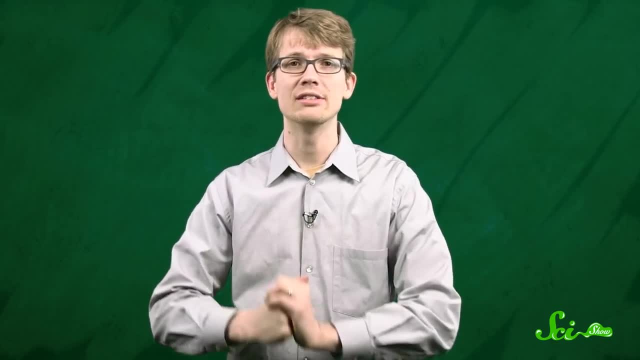 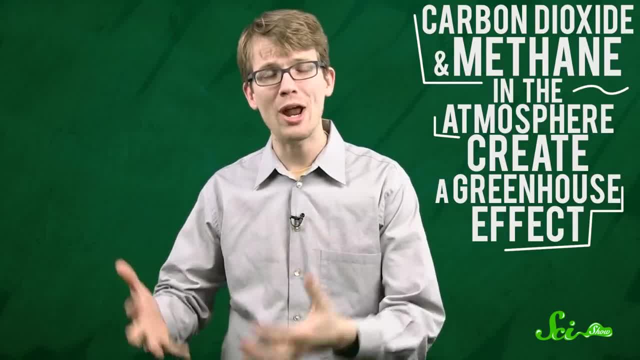 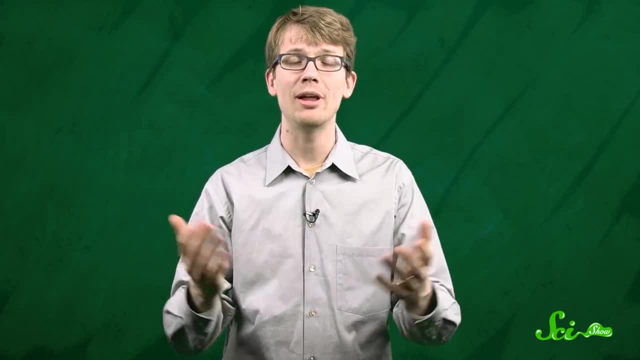 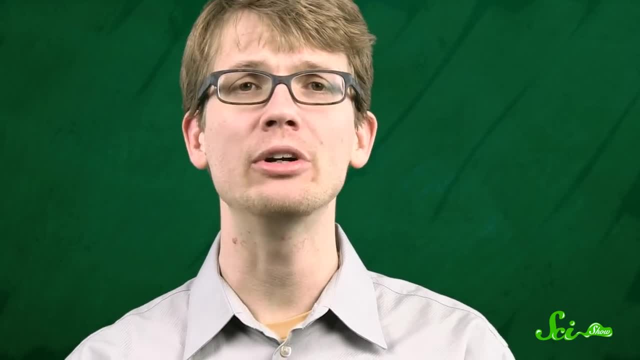 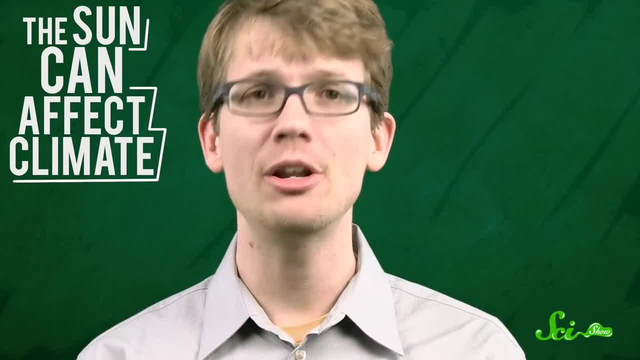 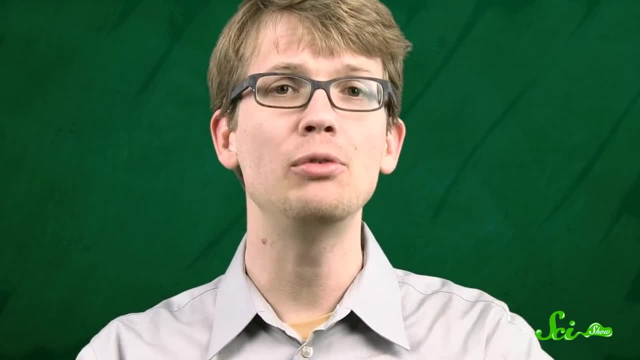 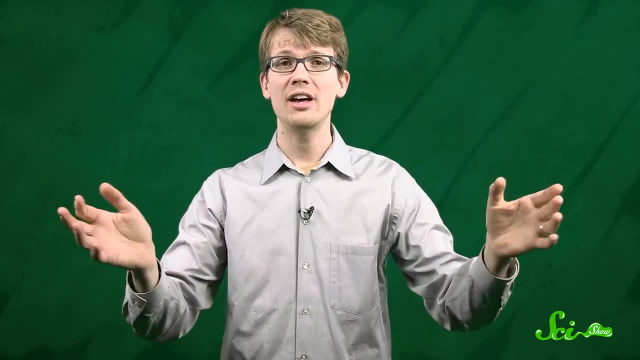 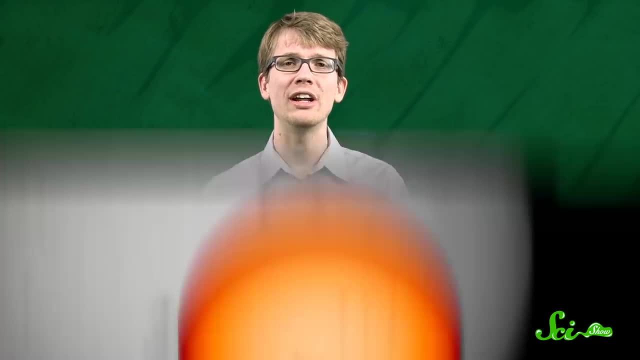 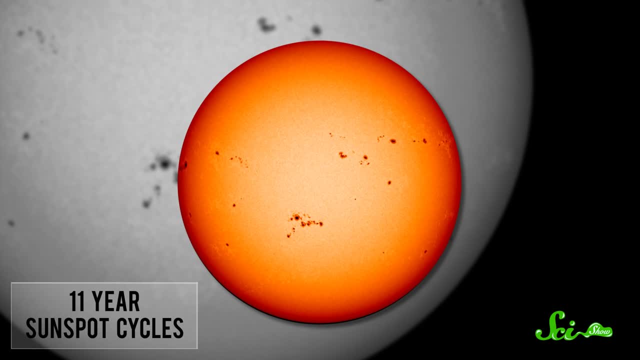 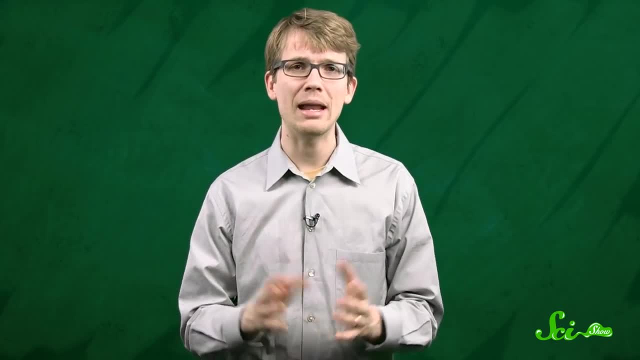 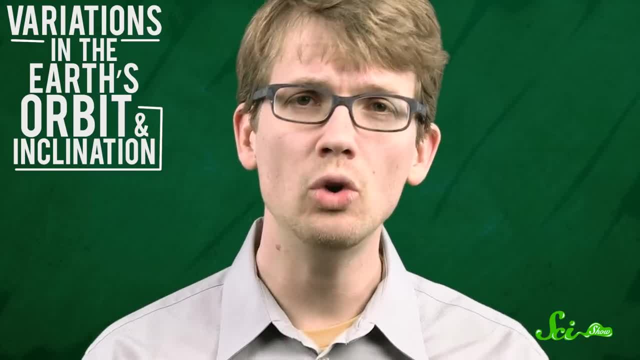 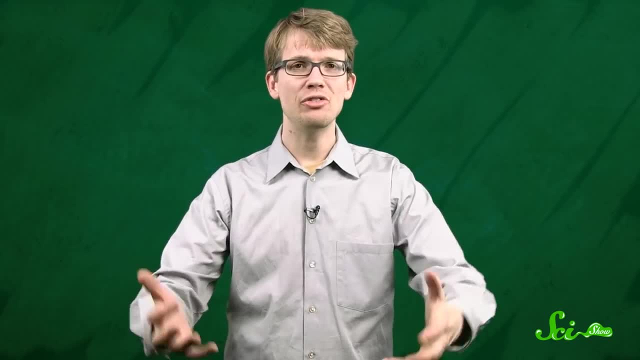 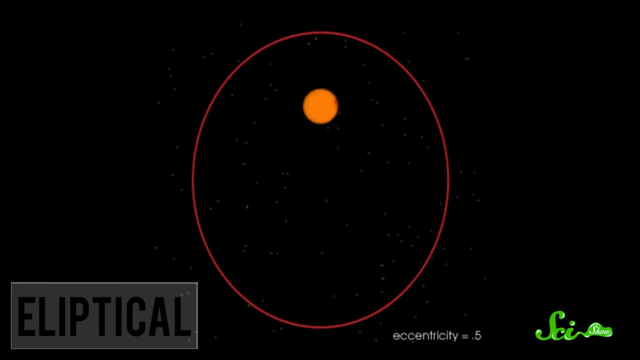 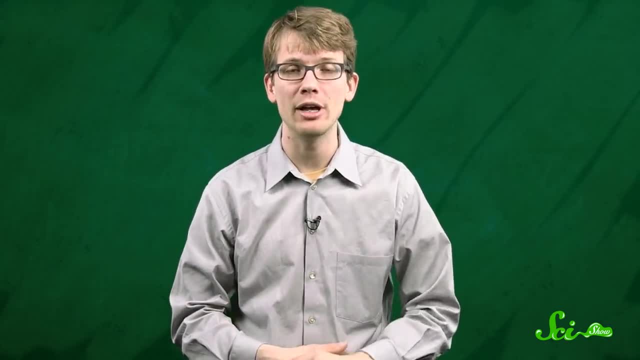 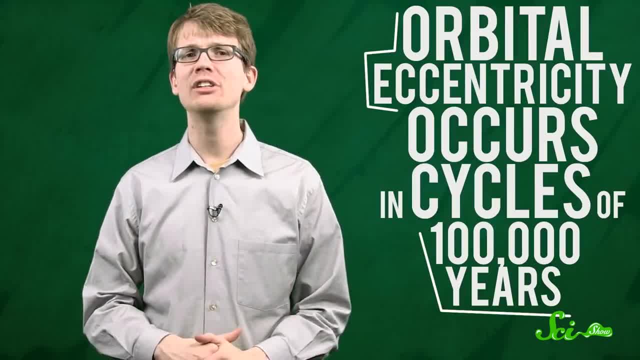 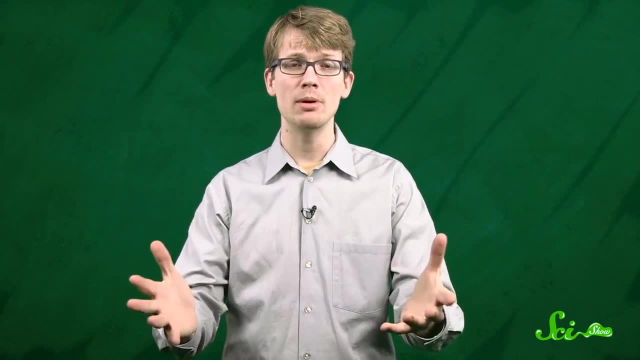 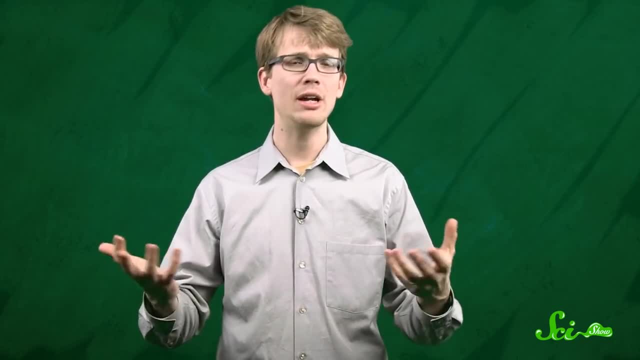 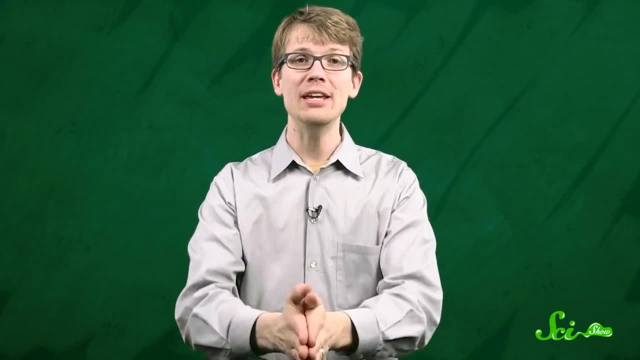 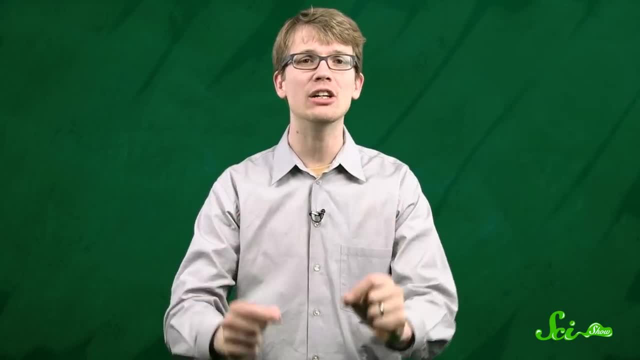 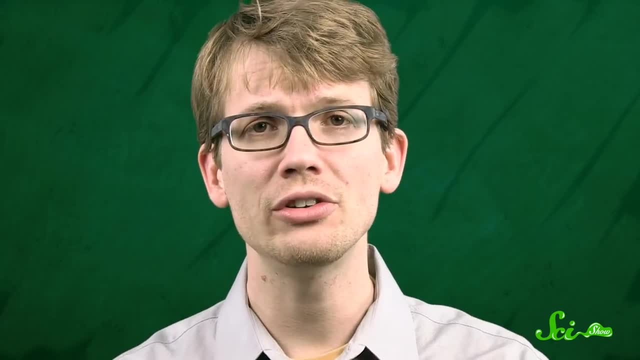 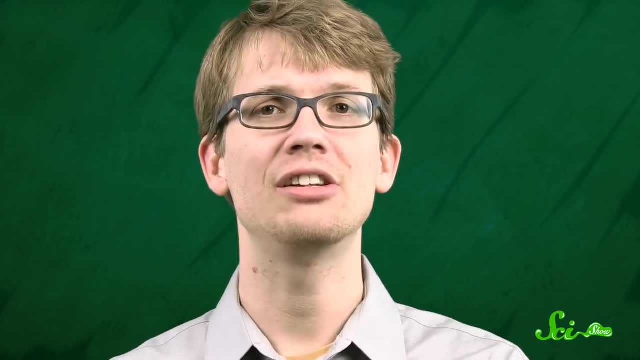 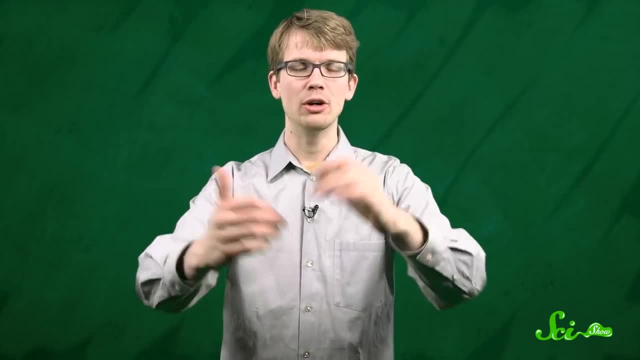 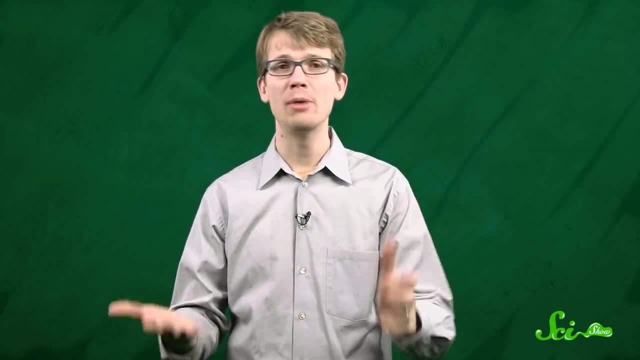 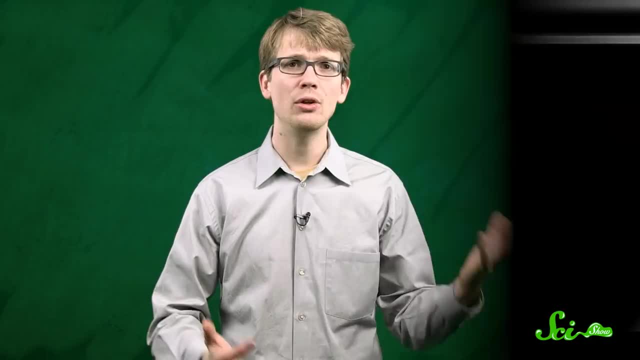 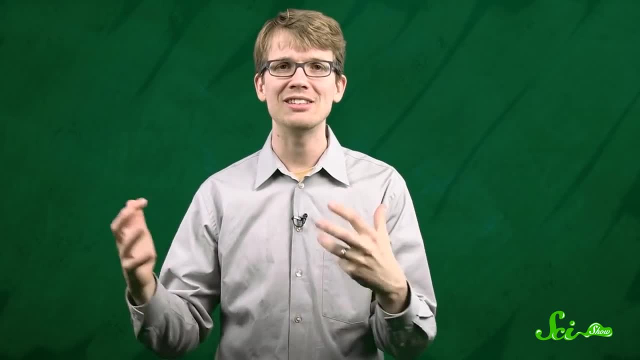 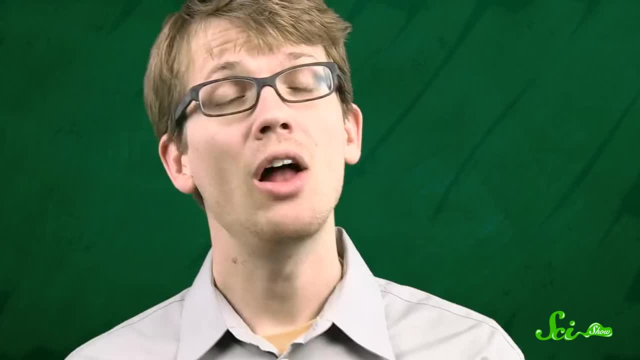 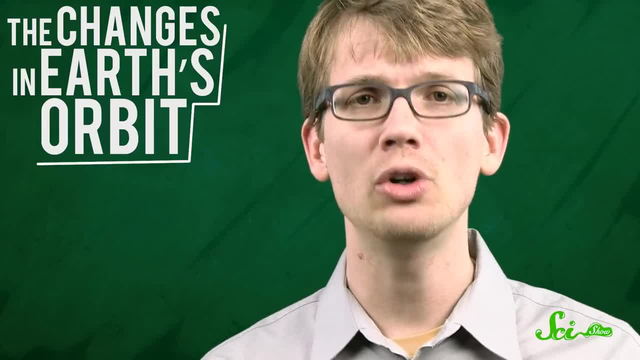 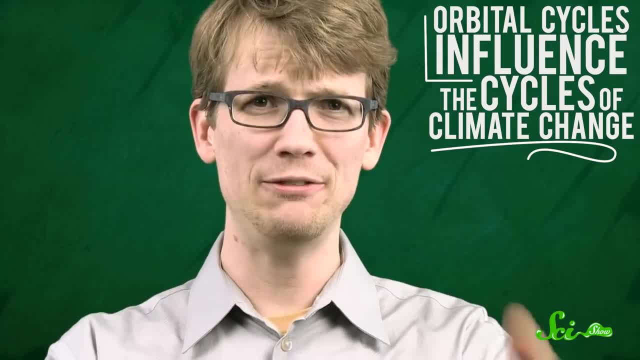 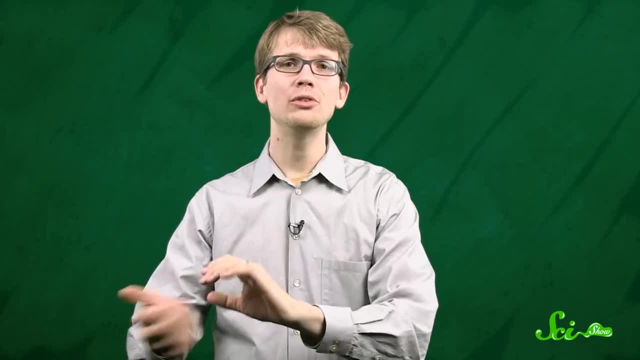 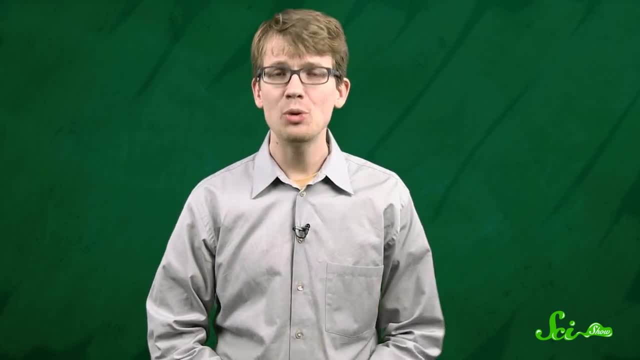 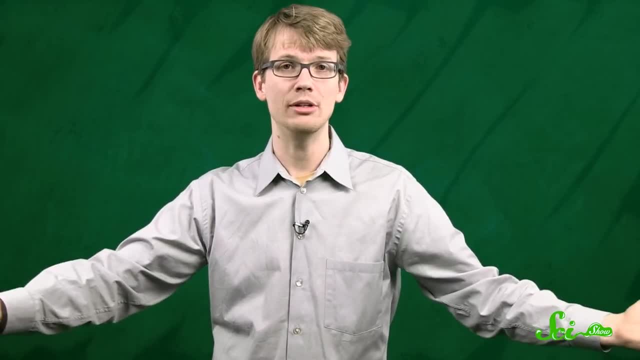 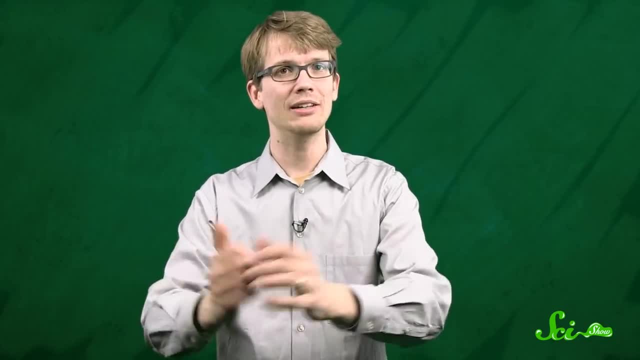 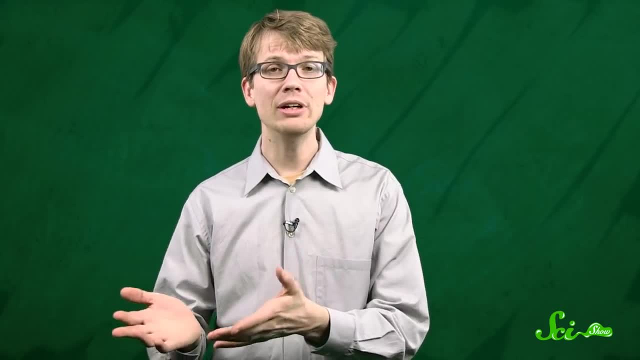 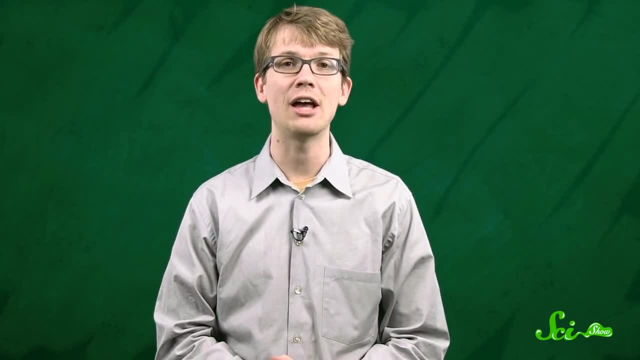 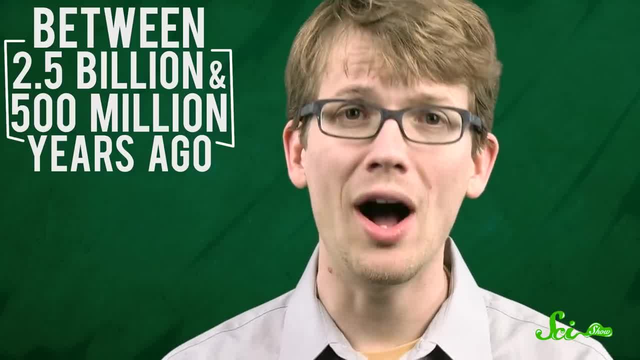 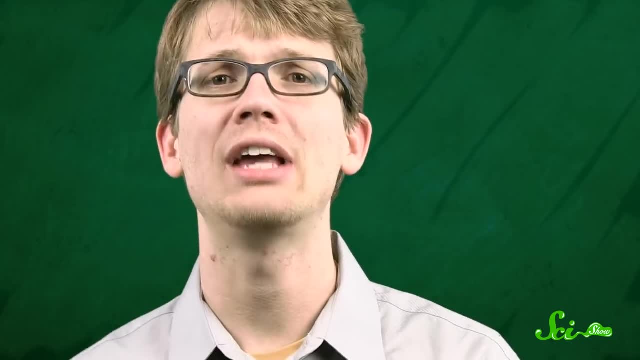 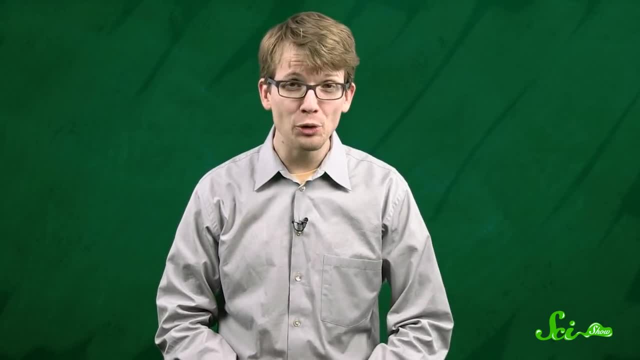 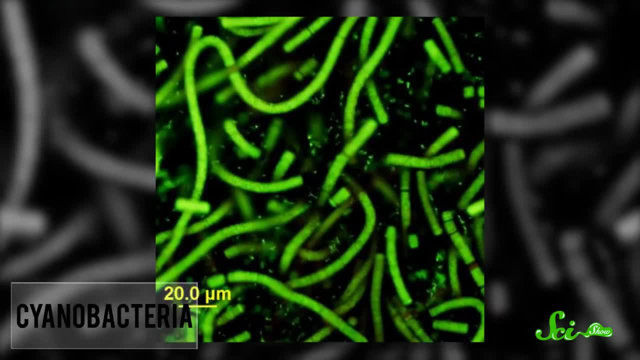 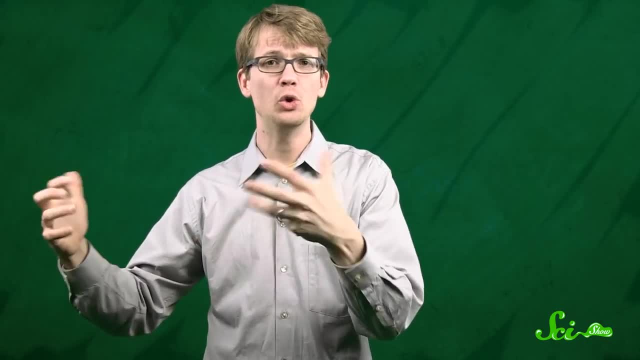 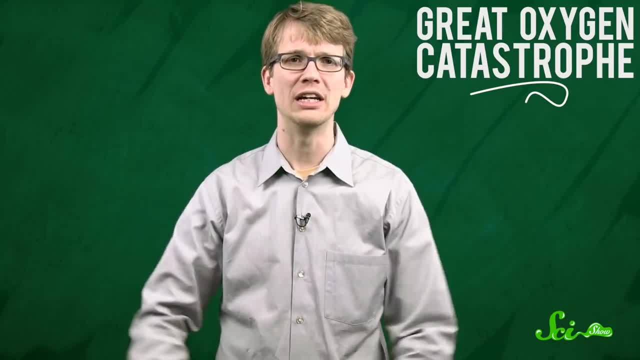 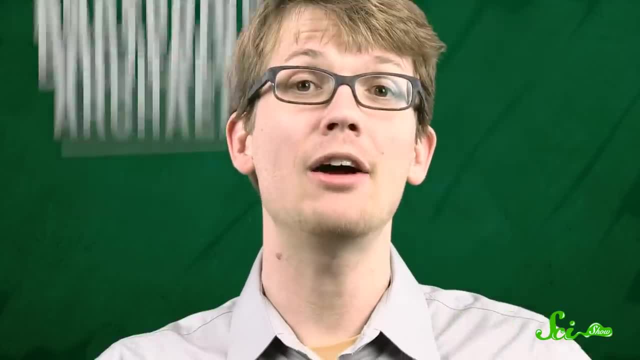 The most recent transition between these two is: the global climate resulted in the Great Oxygen Catastrophe, one of the most significant extinction events in Earth's history. Well, it was the catastrophe of the anaerobic bacteria and the Archaea. but a nice bit of. 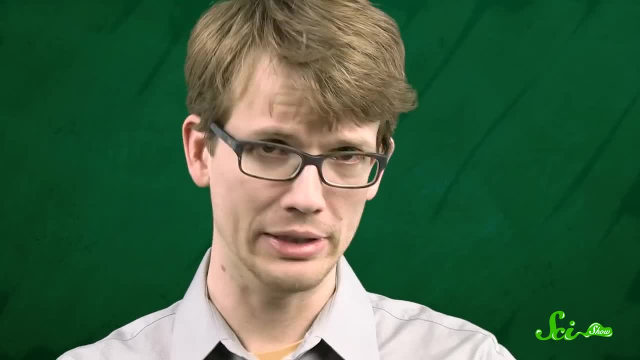 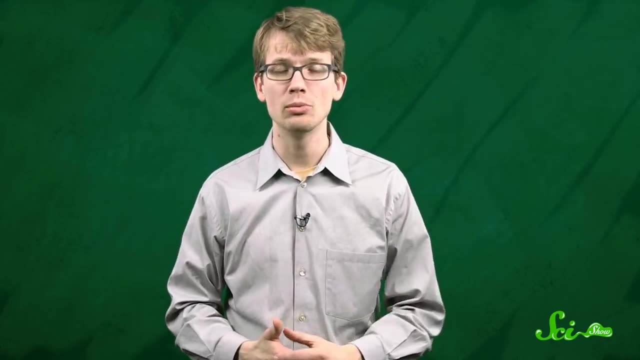 luck for us who wouldn't happen along for another couple billion years or so. I guess it's all about perspective. There was probably a big cooling around this time too, partly because of the rise in oxygen and most of the methane being removed from the atmosphere. At the peak of this cooling period, it's thought that the average temperatures at the equator were about what they are in modern-day Antarctica. Some scientists think that the entire globe essentially froze, resulting in what they call a snowball Earth. Between 500 and 250 million years ago, the planet's core cooled down to the temperature. 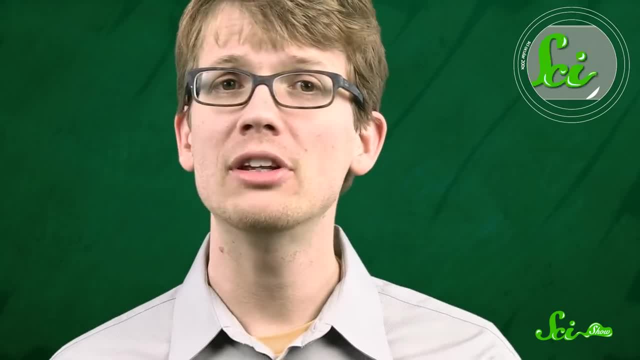 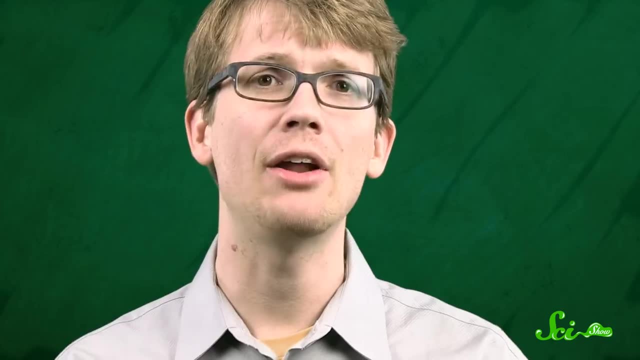 it is today, so volcanic eruptions became rare. It's during this time that we see the Cambrian Explosion, where multicellular life evolved like crazy in the oceans. Photosynthetic organisms on land churned out oxygen, but there weren't yet enough aerobic. 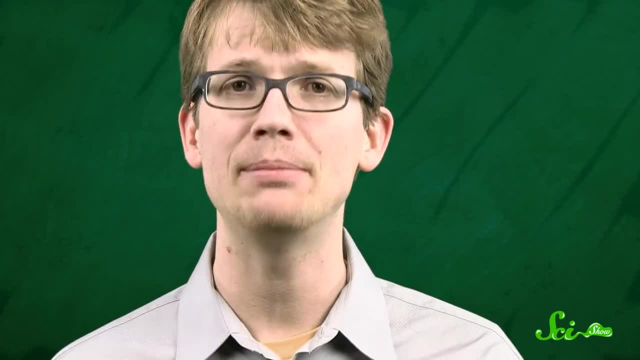 organisms to breathe it in and pump the CO2 back out. so Earth stayed pretty chilly 250 to 65 million years ago. all that changed. By then the Earth would have been completely frozen. By then the Earth would have been completely frozen. 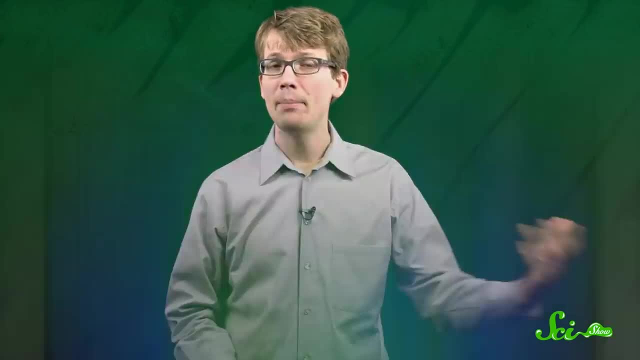 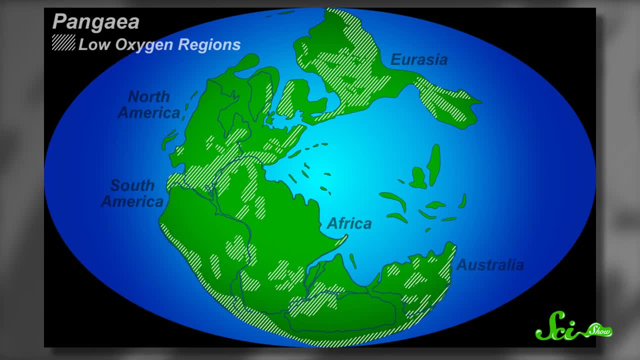 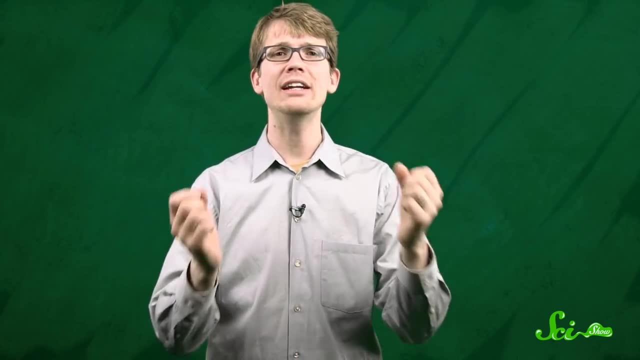 Pangaea, the huge honking supercontinent, was also starting to break up, so more land was coming into contact with the oceans, increasing humidity and helping drive the climate into a warming period. This culminated in a time when temperatures were about 10 degrees Celsius higher than. 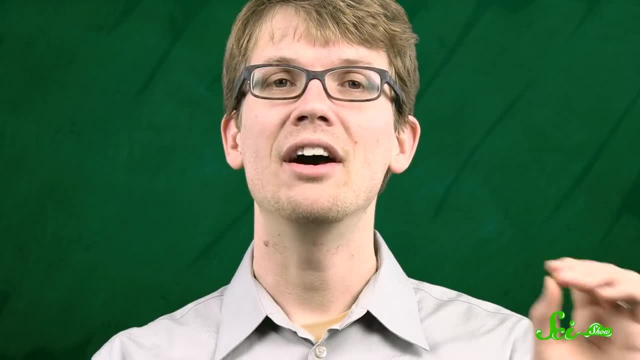 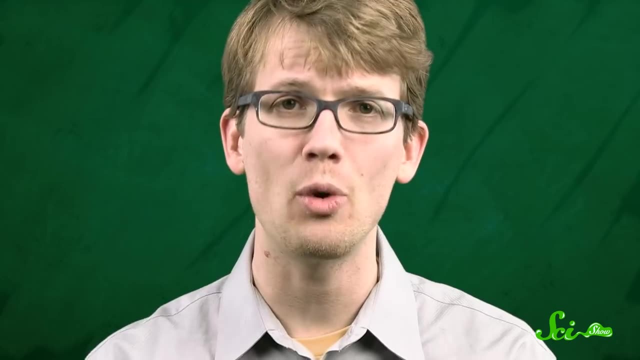 they are today and pretty uniform all over the globe. Then another climate change driver intervened. The reigning theory is that 65 million years ago, a 200-kilometer-wide asteroid smashed into what is now Mexico, spraying up 9 million tons of CO2.. 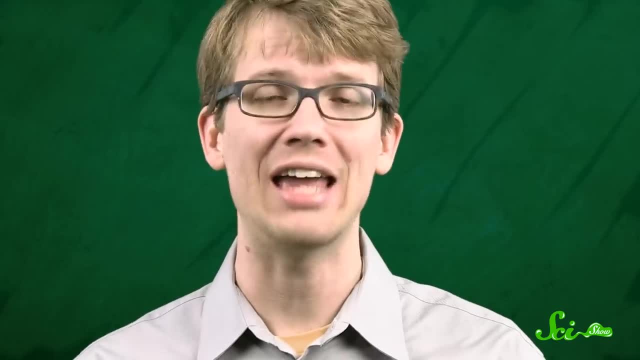 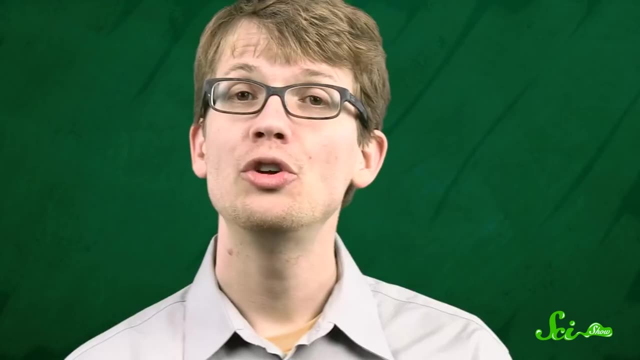 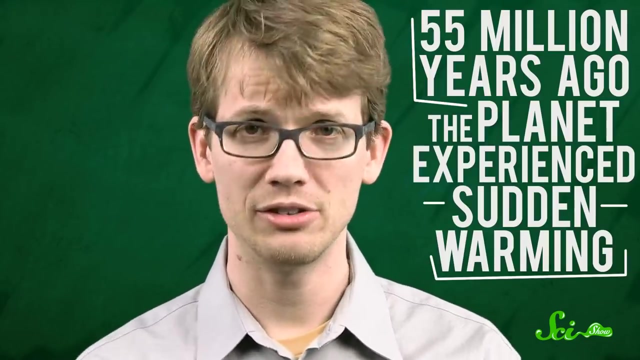 This probably caused an impact winter that was likely enough to kill off all the large dinosaurs and allow mammals to kind of take over. Just 10 million years later, we began the run-up to that thermal maximum I mentioned earlier. About 55 million years ago, the planet experienced sudden warming, which sent global temperatures 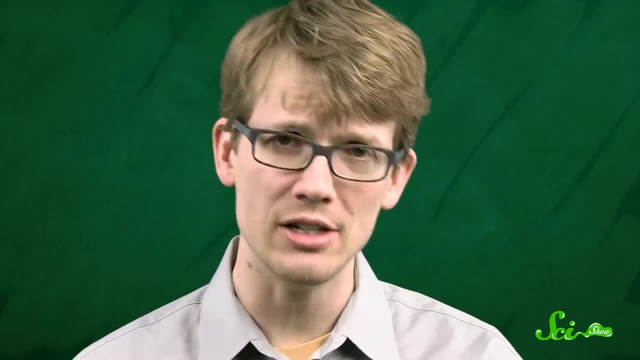 up 5 to 8 degrees Celsius in just 20,000 years. It didn't last very long, and what exactly caused it is a matter of debate, but the geological record shows that there was a huge infusion of carbon dioxide into the atmosphere. 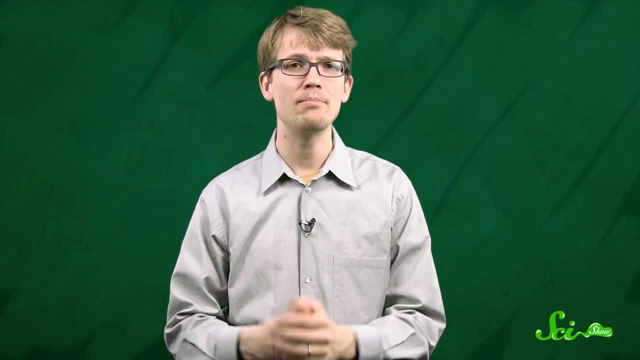 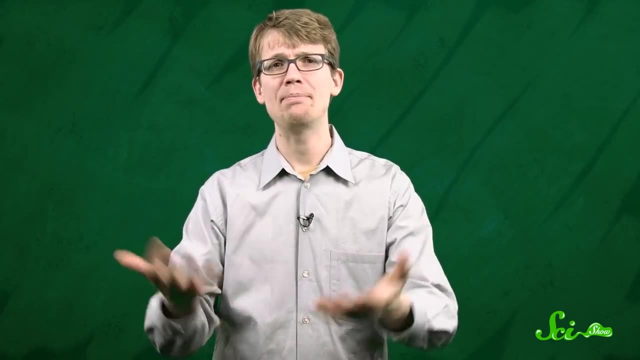 One of the most popular hypotheses is that it came from methane being released, from sudden melting of methane-containing ice under the seafloor and at the poles Something happened, say, undersea volcanic activity or a peak in one of the solar cycles we talked about, to melt this methane ice. 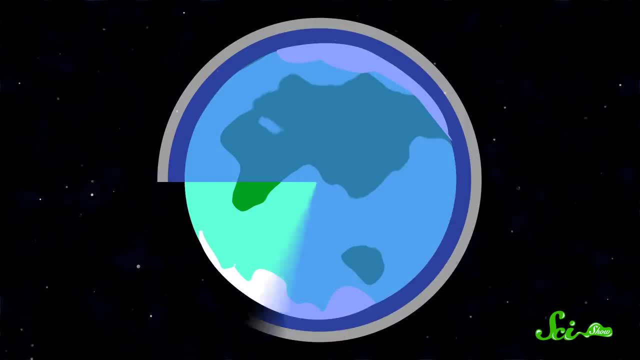 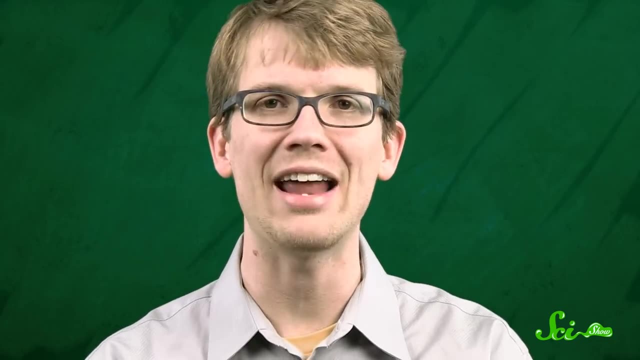 And once it was unleashed into the atmosphere, we were all in Greenhouse City. Because of this little escapade, the Earth went completely ice-free, the opposite of Snowball Earth, sometimes called Greenhouse Earth or Hot House Earth, And, in addition to creating an ideal climate for warm-blooded creatures, the Earth was 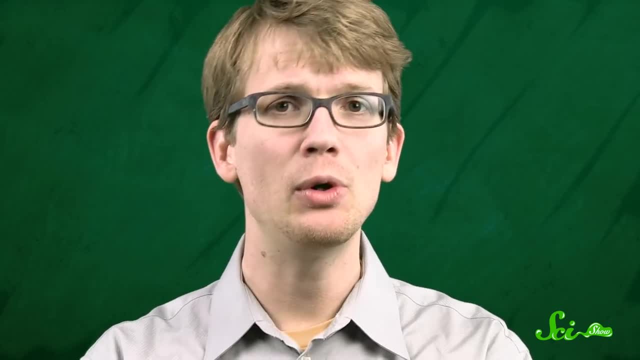 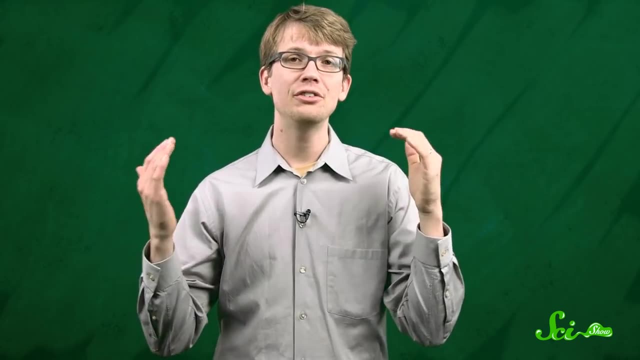 completely ice-free. This also allowed for the proliferation of more plant life, including that huge bloom of a Zola freshwater fern. So levels of greenhouse gases started to tank yet again, but when the next cooling trend began, this time it was different. 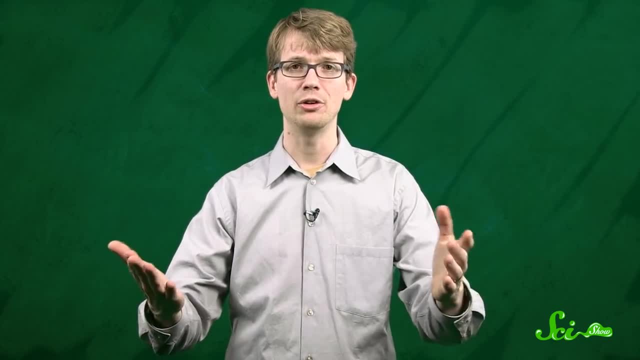 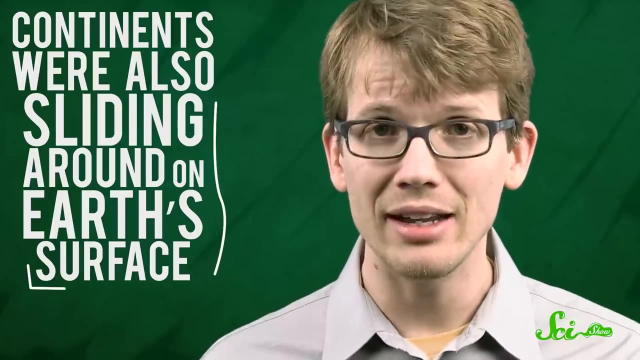 About 35 million years ago, glaciers started to form in Antarctica for the first time, in part because there was no Antarctica before See. while all the cycles that we've been talking about kept churning, the continents were also sliding around on the Earth's surface, until landmasses appeared at the South Pole. 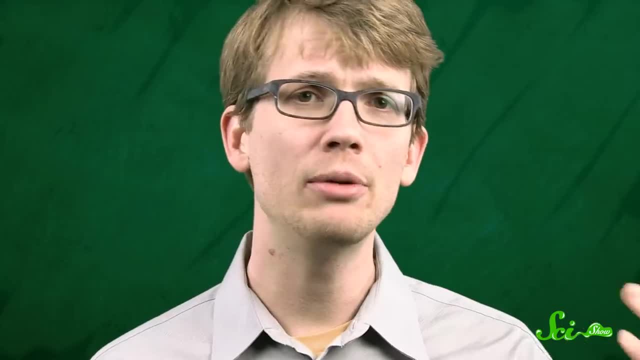 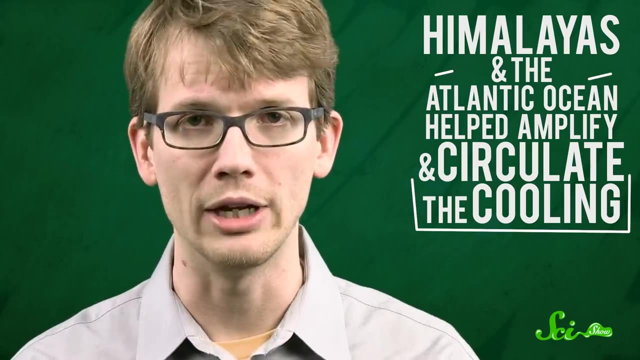 That allowed glaciation to take place. Meanwhile, other formations that didn't exist before, like the Himalayas and the Atlantic Ocean, had taken shape, which helped to amplify and circulate the cooling And thus began a major icehouse climate. When people talk about the Ice Age, this is usually what they mean, and because there's 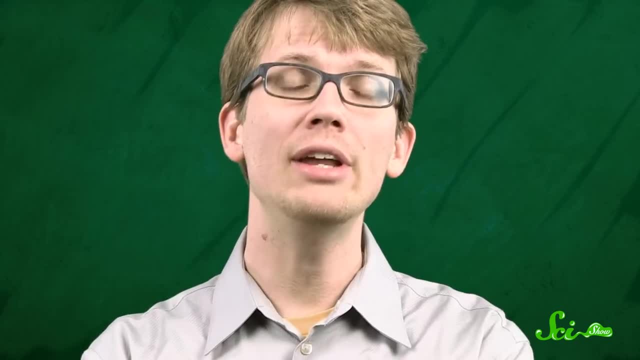 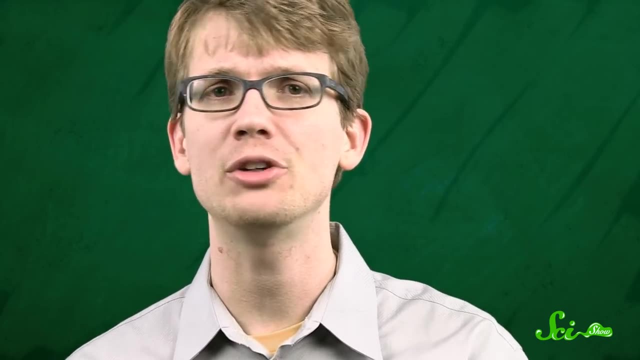 still permanent ice to be found. we're technically still in it, But this cooling hasn't been consistent. Within this ice age, there have been small warming events interspersed with even cooler events where average temperatures were about 5 degrees celsius cooler than today. 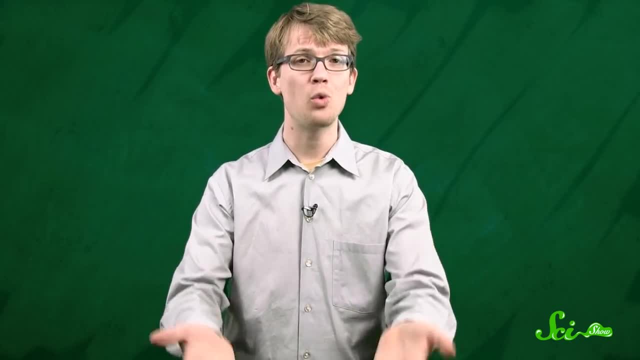 In fact, in the past few years there have been more cooling events. In the past 2.5 million years, there have probably been around 25 glaciations or cold periods, sometimes called little ice ages, interspersed with interglacials, which are 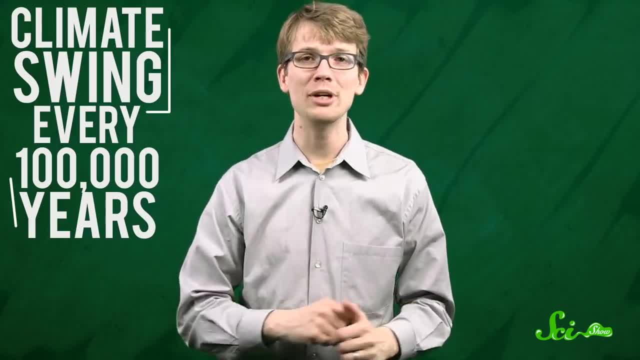 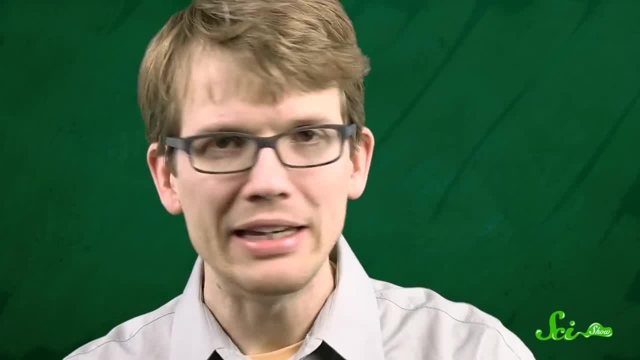 warmer periods. You might notice that that comes out to about one climate swing every 100,000 years, which coincides with that orbital pattern we talked about And that brings us up to now, or, you know, within about 12,000 years of now, which is 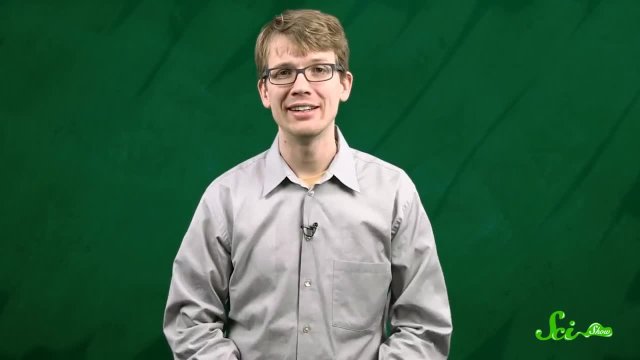 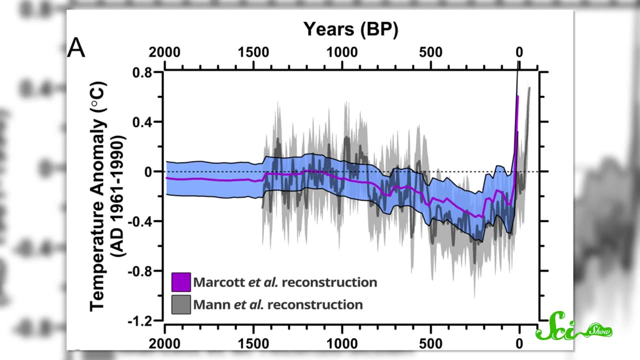 like yesterday in geologic time. So you've heard of the hockey stick, right? It's this graph depicting the average global temperatures over the last 2,000 years or so, based on what can be gathered from historical data: tree rings, corals and ice cores. 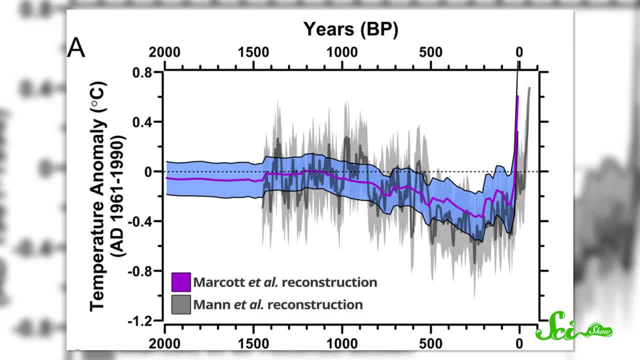 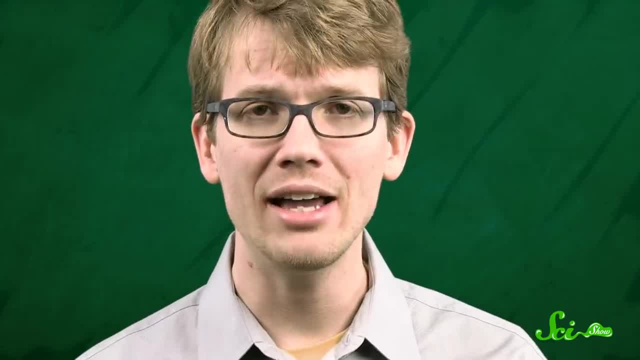 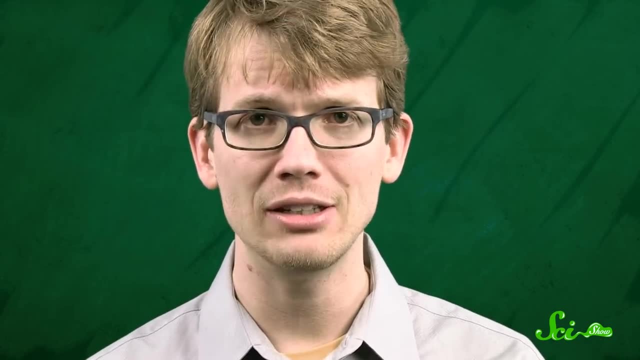 You'll notice that average temperatures increased dramatically during the 20th century, which is when we started relying heavily on fossil fuels to power our everything. This graph came out in 1999, using data collected by Penn State climate scientist Michael Mann, who has taken an incredible amount of heat for this research over the past 15 years. 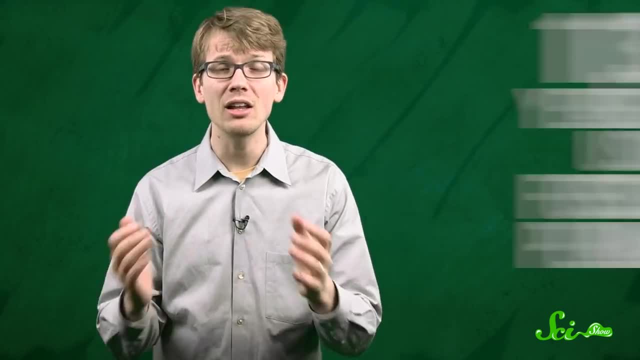 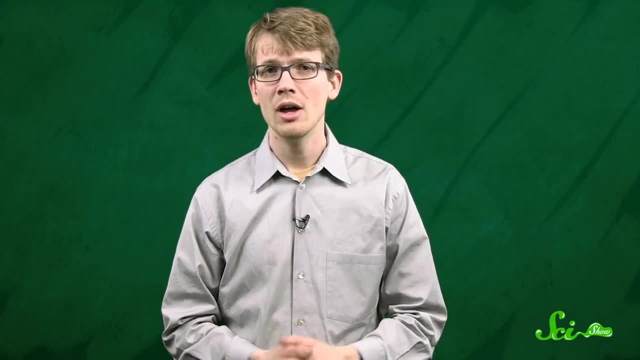 But new research reconstructs global temperatures further back than Mann did, 11,300 years back using fossilized plankton dug up by oceanographers from 70 sites worldwide. On one hand, it shows that temperatures for about 20% of this historical period were actually 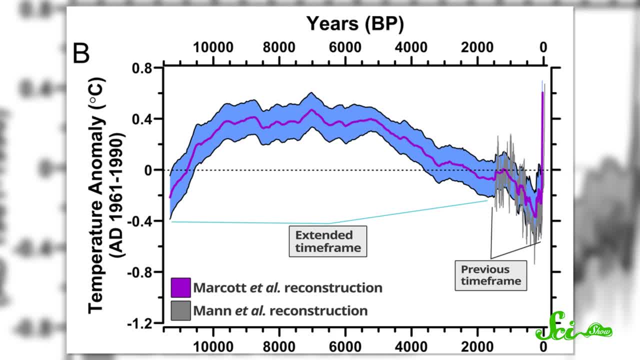 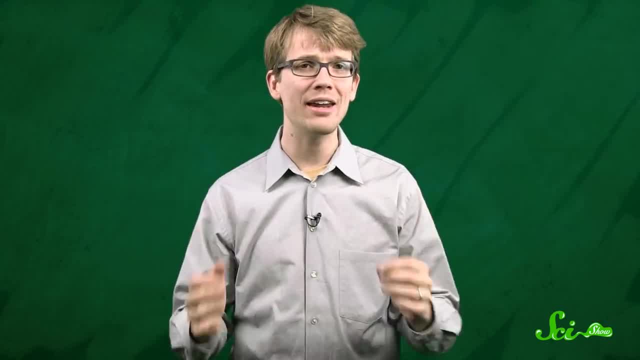 higher than they are today, But it also shows that right now, temperatures are increasing faster than they ever have In the past 100 years. temperatures have risen so dramatically that they have canceled out all of the cooling that took place over the past 6,000 years. 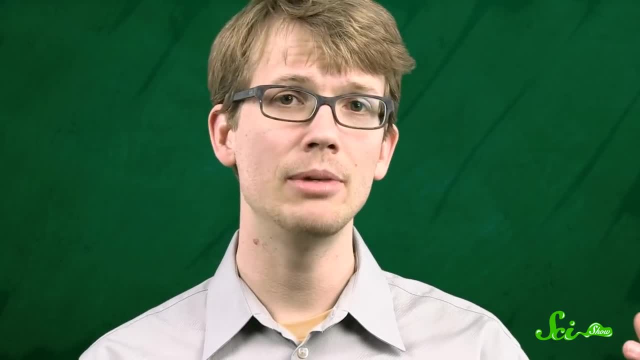 And probably more important. the study shows that, in addition to being in the middle of a long-term ice age, we should be able to see the temperature rise and fall. We should be able to see the temperature rise and fall. We should be able to see the temperature rise and fall. 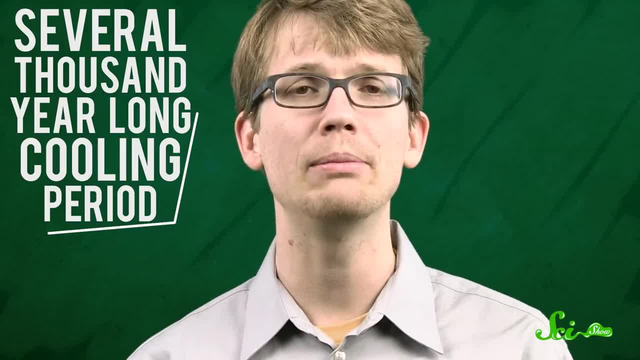 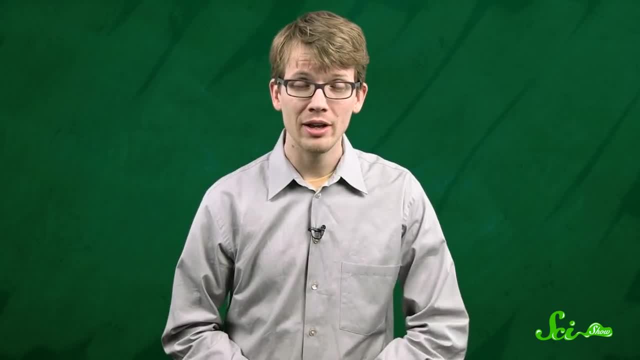 We should now be entering the bottom of a several-thousand-year-long cooling period, even if it were just natural factors, But it's not So. this new evidence pretty much corroborates what's already known- that we're making a mess. But one thing's for sure: our planet's climate has dealt with a lot, and it'll probably 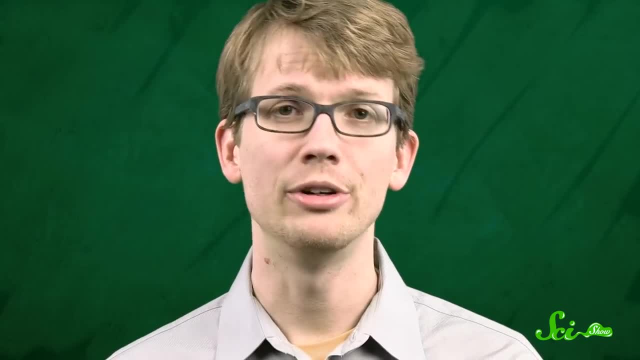 survive humans, But what the cost will be for us. we're going to need some more data on that. Thanks for watching this episode of SciShow. If you have any questions, comments or suggestions for us, you can find us on Facebook and Twitter. 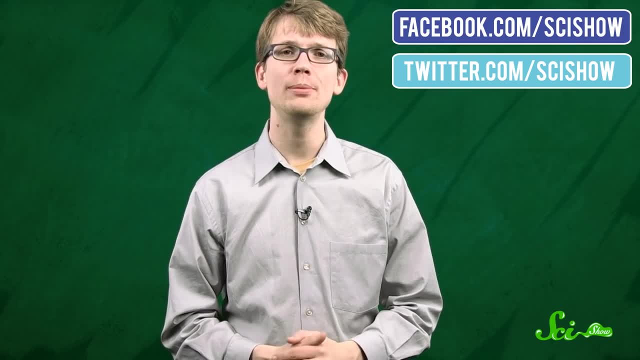 or down in the comments. And if you want to keep getting smarter with us here at SciShow, you can go to youtubecom, slash scishow and subscribe.